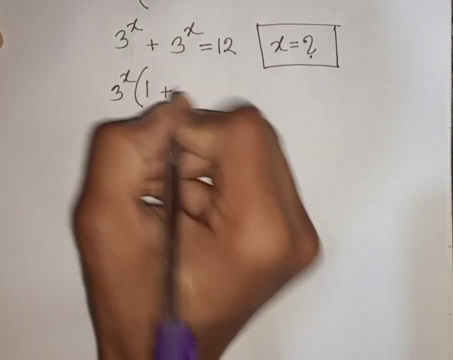 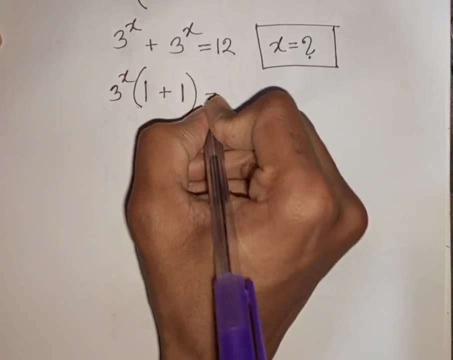 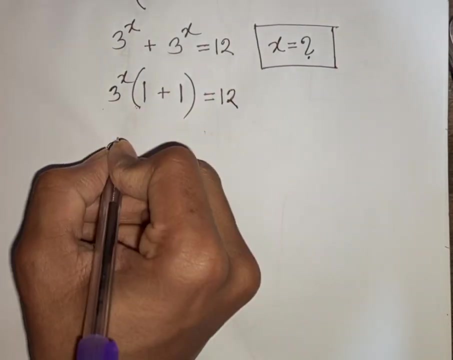 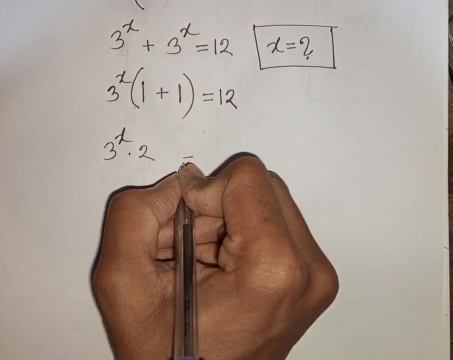 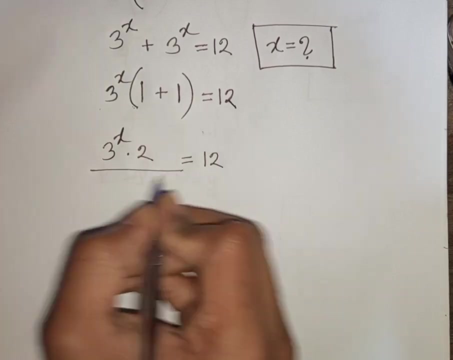 this: that means it will be on plus this. divided by this, that means on, Then bracket close is equal to 12.. Now we have 3 power x times 1 plus 1. that means it will be 2 is equal to 12.. Now we divided by 2 in both sides, So divided by 2, divided by 2.. So this 2, this 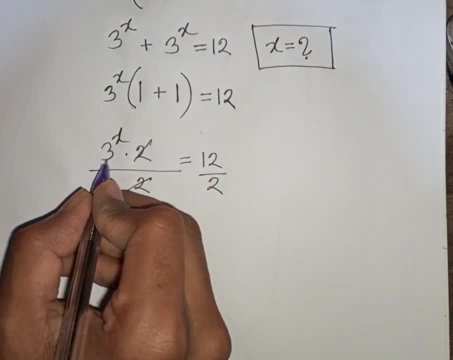 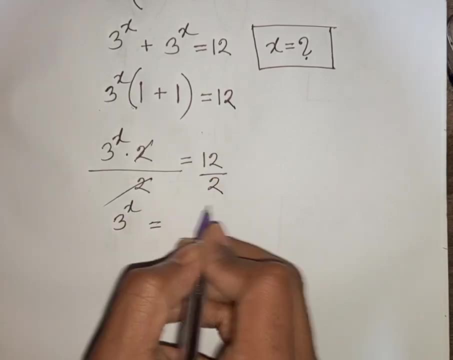 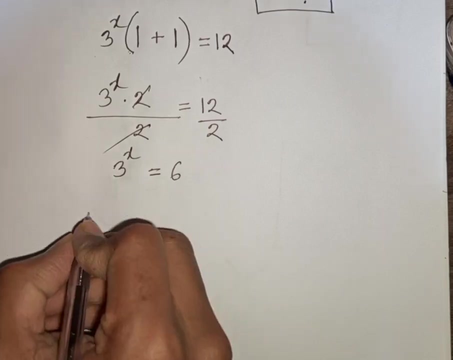 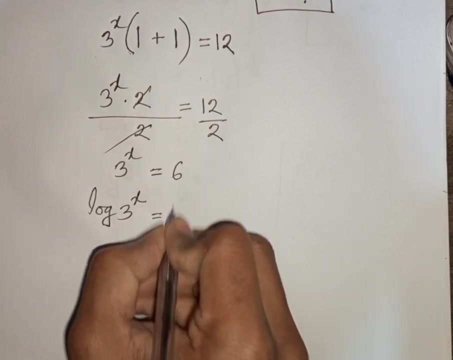 2 will be cancelled. Now we can write here: 3 power x is equal to 12 divided by 2, that means it will be 6.. Now we apply log in both sides So you can write here: log of 3 power x is equal to log. 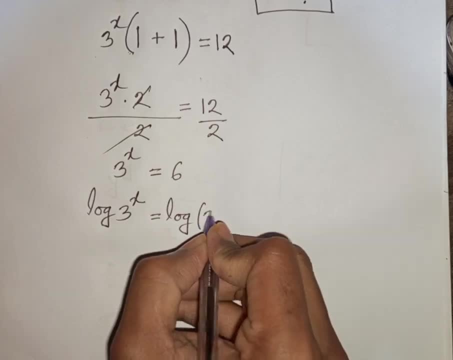 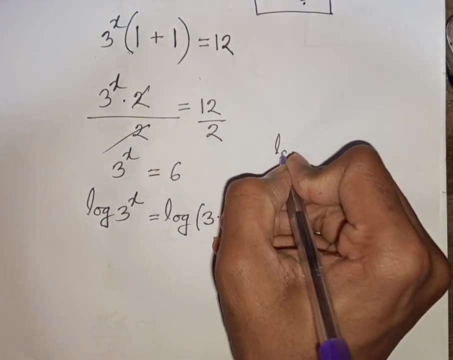 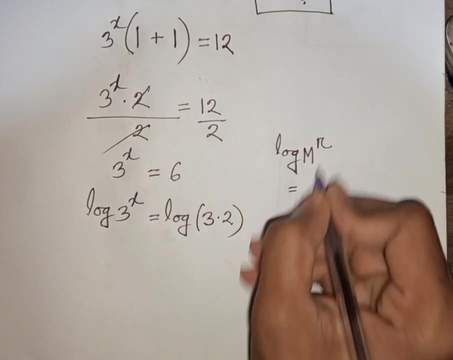 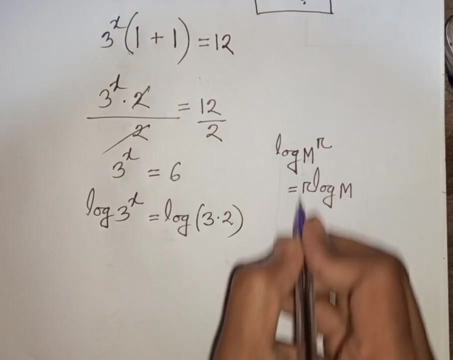 of 6 can be written as 3 times 2.. Now here we can apply rule that log m, power r is equal to r log m. That means this power r moved to the base. So according to this rule we can compare here this power x will. 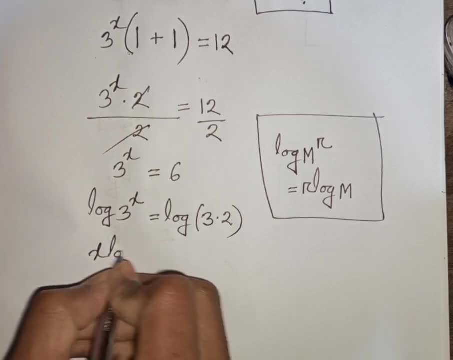 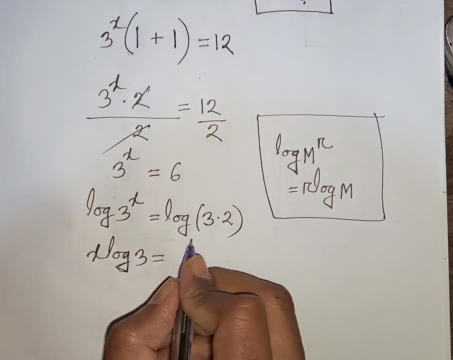 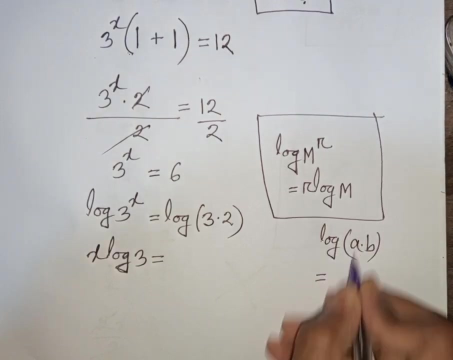 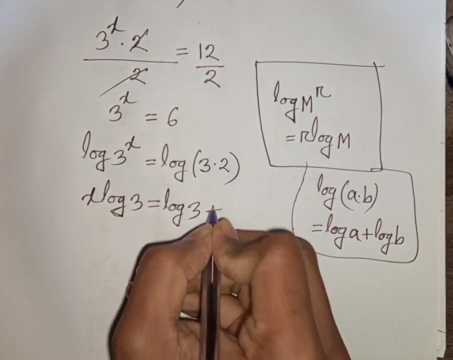 move to the base. So you can write here: x, log m, power. r can be written as r, So this you can look like that 3 is equal to. here I can apply this formula: log of a times B is equal to log a, log a plus log b. So according to this formula, we can write here: log 3 plus log 2.. 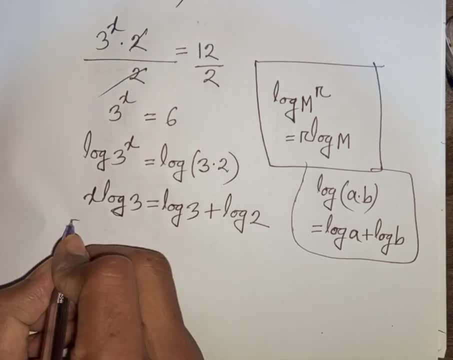 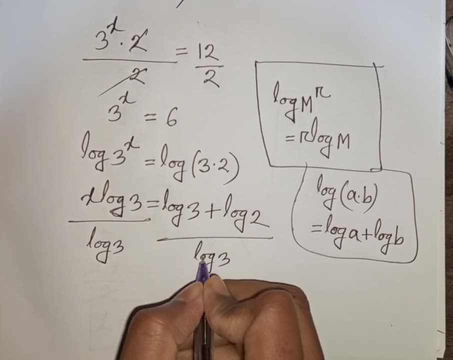 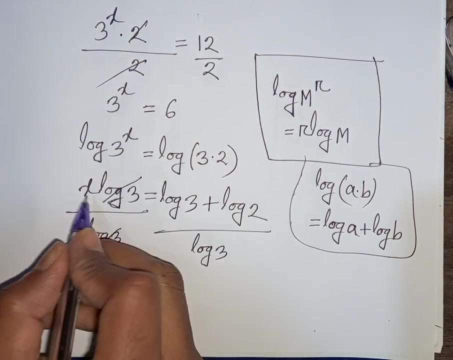 Now we need the value of x. so we divide it by log 3 in both sides. so divide it by x, x log 3 divided by log 3.. Now this log 3, this log 3 will be cancelled, So here x will.